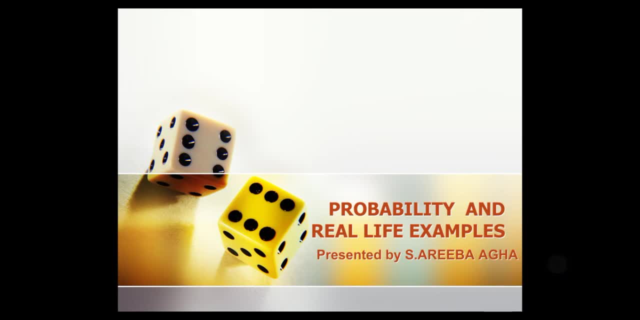 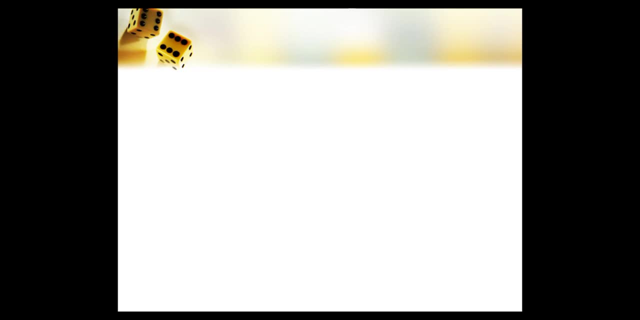 Assalamu alaikum, this is Sayyeda Reba Agha, and my topic is probability and real life examples. What is probability? The chance something will happen, or how likely it is that an event will occur? For example, in sports, we toss the coin and both teams have 50 over 50 chance of winning it. 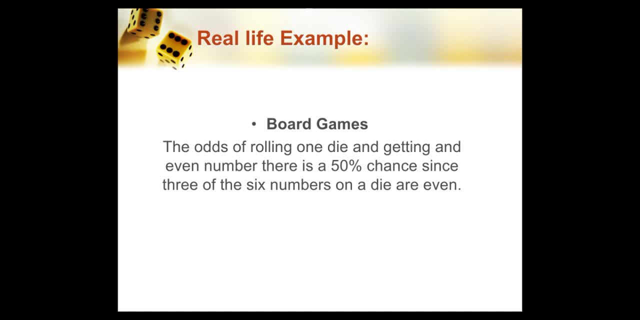 In board games the odd of rolling one die and getting one event number. there is 50% chance. since three of the six numbers on a die are events In medical decisions. when a patient dies, the odds are 50 over 50.. 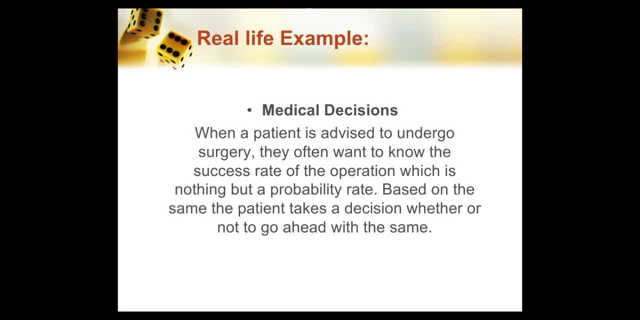 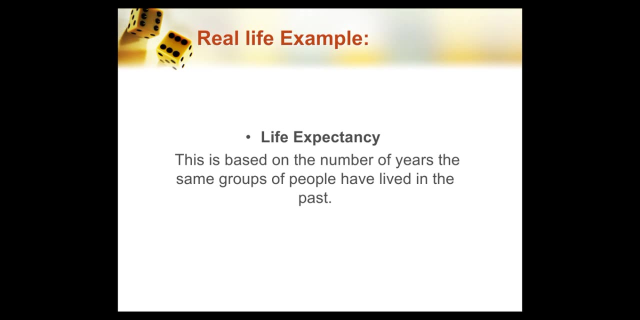 What is probability, The chance something will happen, or how likely it is that an event will occur? When a patient is advised to undergo surgery, they often want to know the success rate of the operation, which is nothing but a probability rate. Life expectancy: this is based on the number of years and the same group of people having lived in the past. 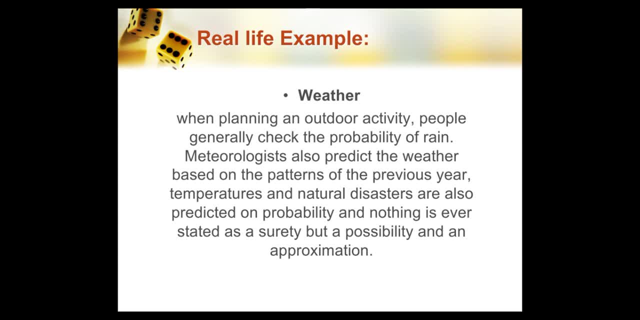 Weather. when planning an outdoor activity, people generally check the probability of rain. Meteorologist also predicts the weather based on the pattern of weather. The natural disasters are also predicted on the probability and nothing is ever stated as surety but a probability and approximation. 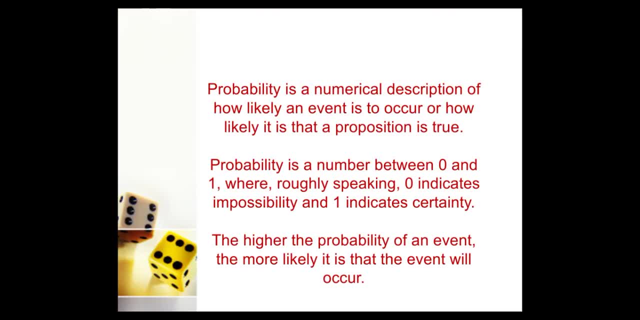 Let's conclude. Probability is a numerical description of how likely an event is occur or how likely it is that a position is true. Probability is a number between 0 and 1, where, roughly speaking, 0 indicates a probability. What is probability? Probability is a number between 0 and 1, where, roughly speaking, 0 indicates a probability. 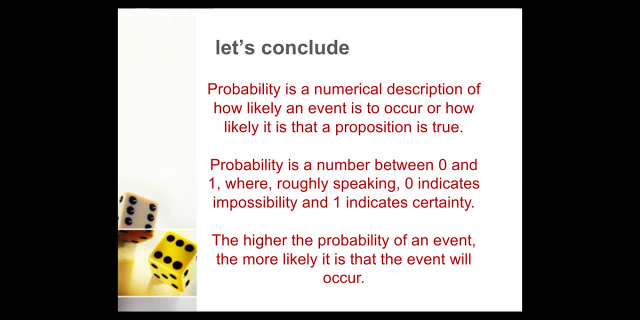 What is probability? Probability is a number between 0 and 1, where, roughly speaking, 0 indicates a probability and one indicates satanism. In the last we said that the higher probability an event is, the more likely it is that an event will occur. 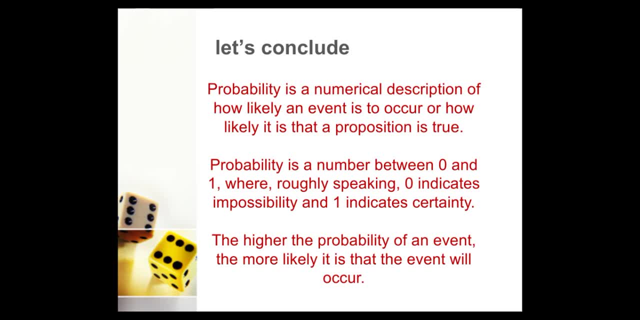 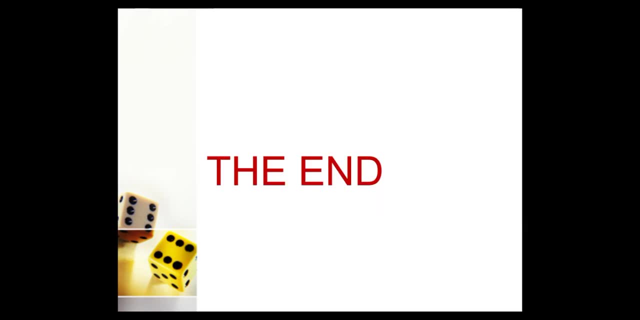 In the last we said that the higher probability an event is, the more likely it is that an event will occur. Thank you,